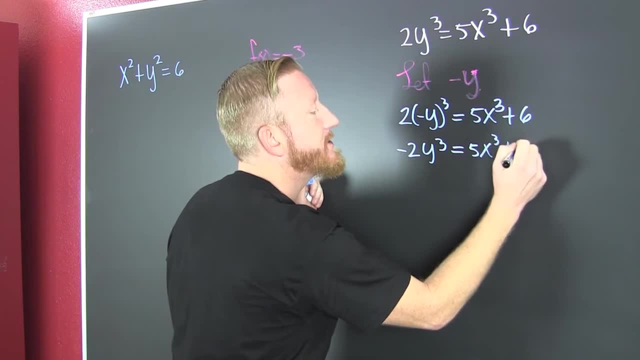 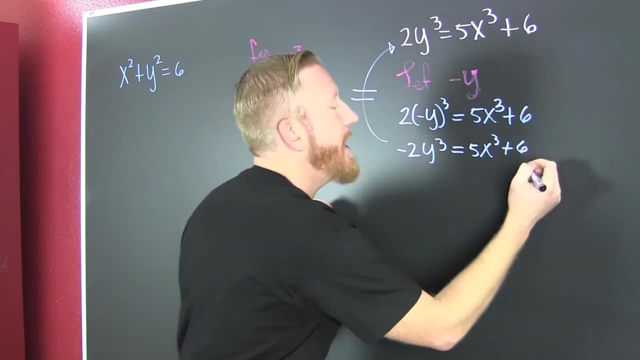 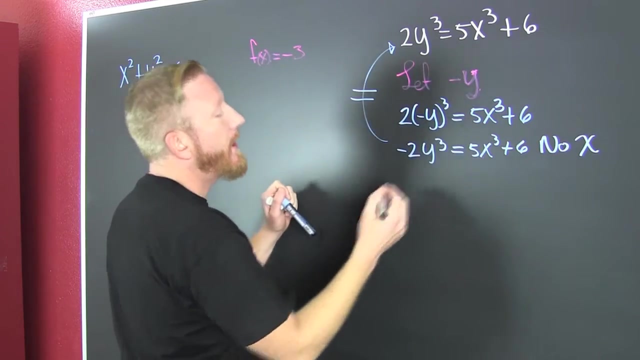 is 5x to the third plus 6.. Now we check: Is this the same? Oh, you are not the same. So it is not x-axis symmetry. Then we go and we check to see if y For y-axis symmetry. 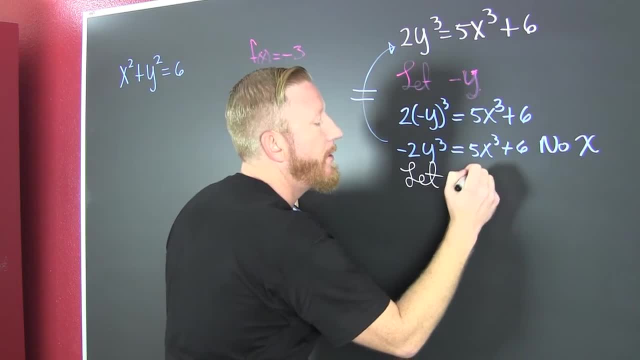 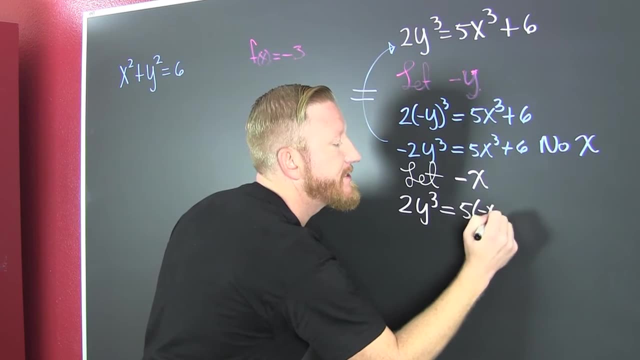 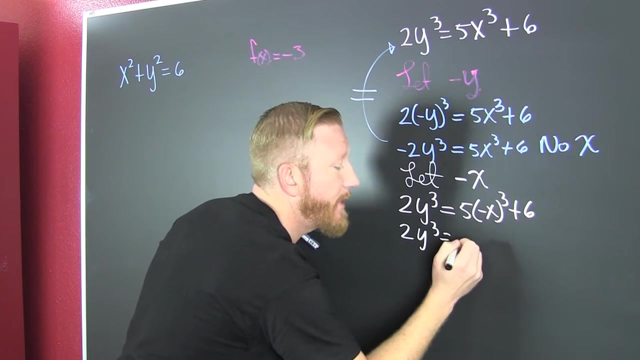 we let a minus x and we put it in there. That's 2y to the third. That's 5 times a minus x to the third, plus 6.. That's 2y to the third. That's going to be. it's an odd power, So. 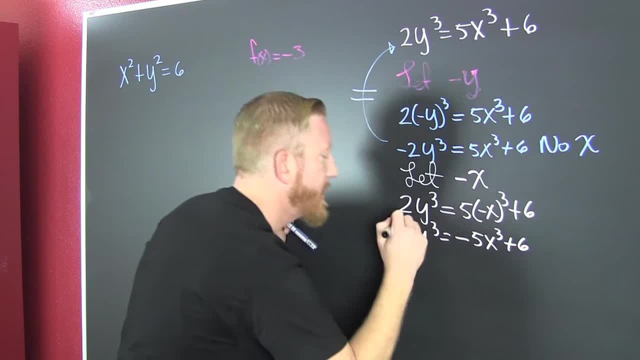 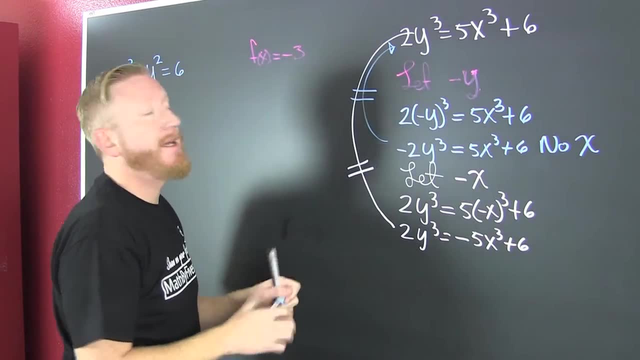 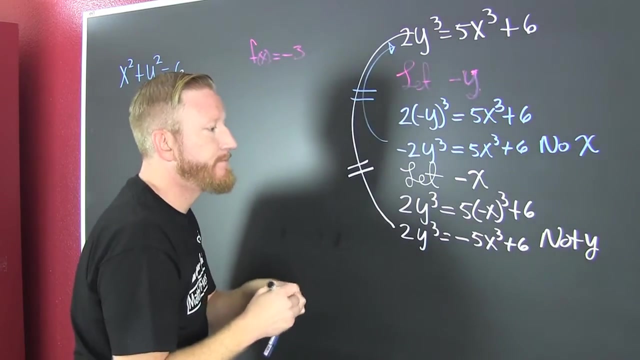 that's minus 5x to the third plus 6.. Are these the same? No, That's not equal. Now one more time. So for origin, Let's check for origin. So it was not y. So for origin, for origin. 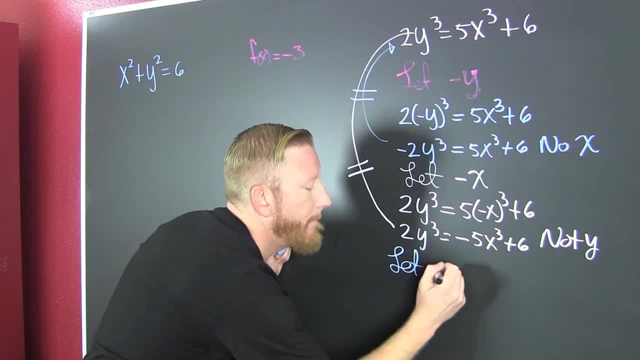 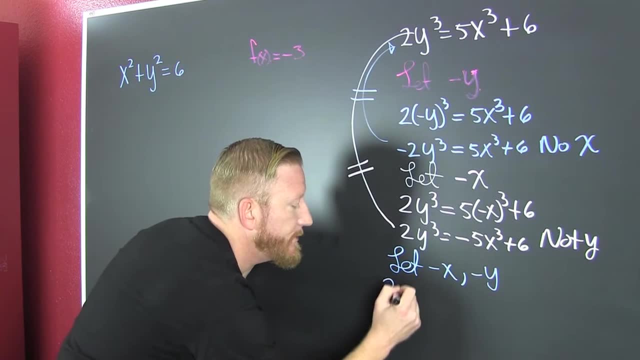 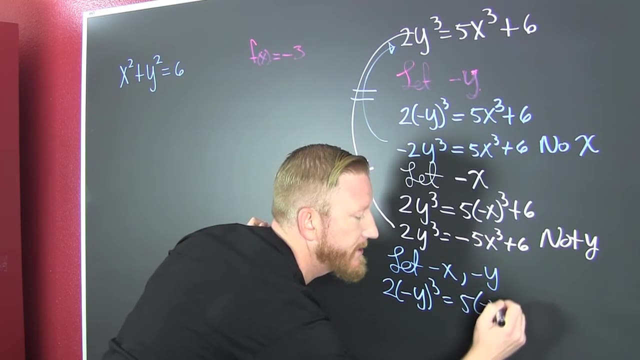 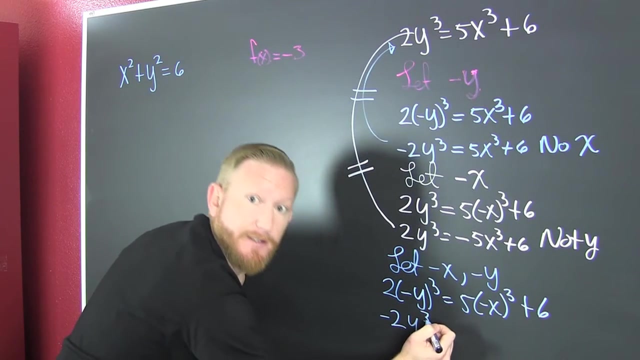 Alright, We are going to let minus x and minus y, So we are checking that guy, Alright? So then that's two times minus y to the third. That's five times a minus x to the third, plus six. So what? Minus 2y to the third. 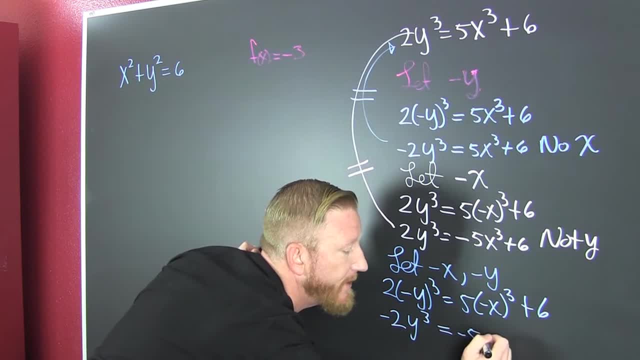 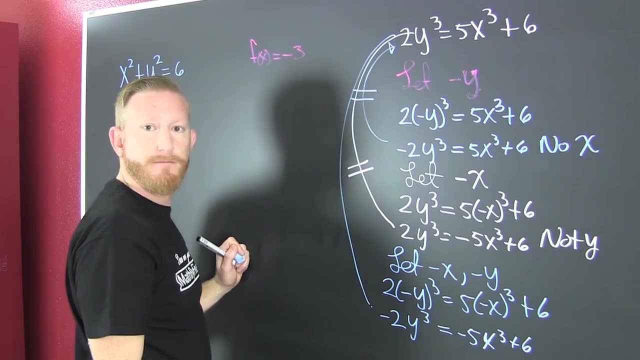 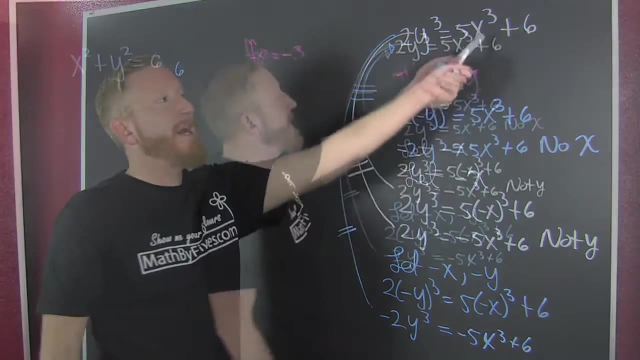 Can you? Yeah, we're good. And a minus 5x to the third, plus 6.. Are these the same? No, They're not the same. Because of that plus 6, we can't get rid of that minus sign. 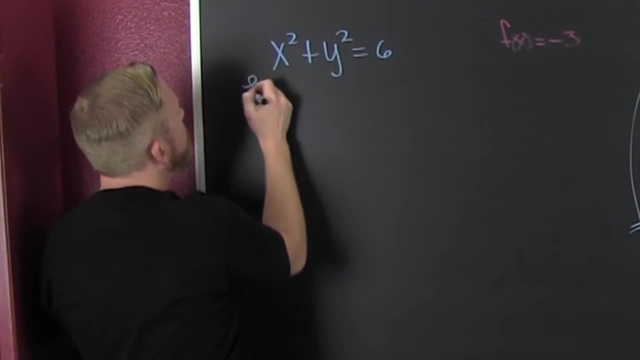 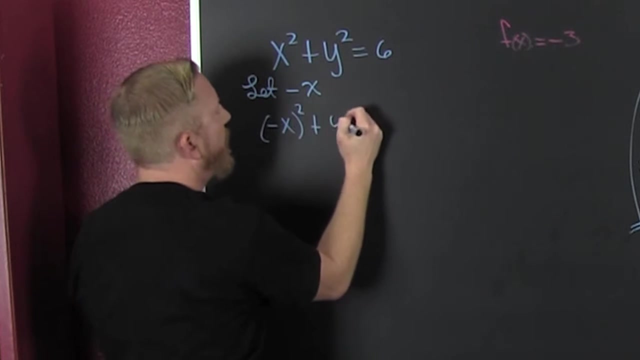 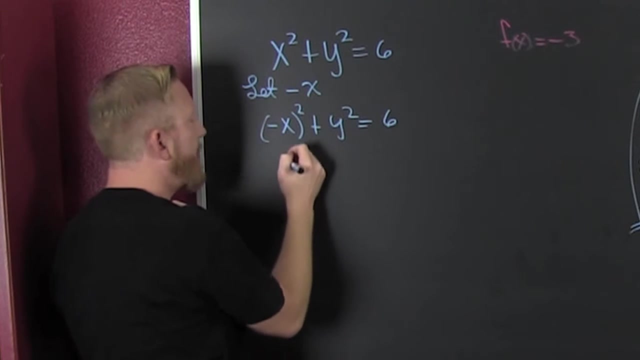 Now let's go and look at this. Let's let a minus x happen, So I put a minus x squared plus a y squared, That's 6.. Okay, That's an even power. So it's minus x times minus x, which is x squared plus y squared. 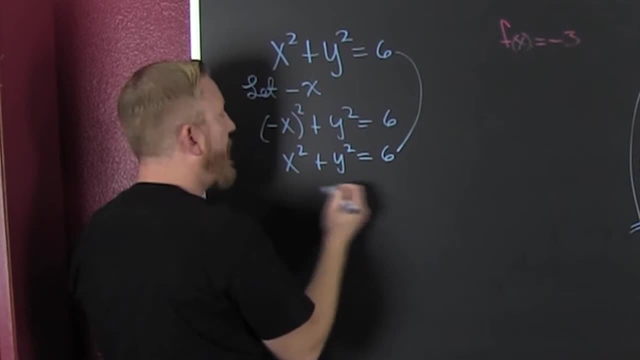 That's 6.. Are these the same? Yeah, So this is y symmetric. All right, Let's check x. Check x symmetry. So we let a minus y happen. So I put a minus y up in there. 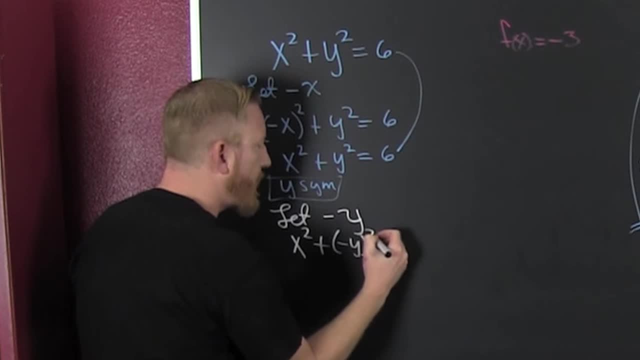 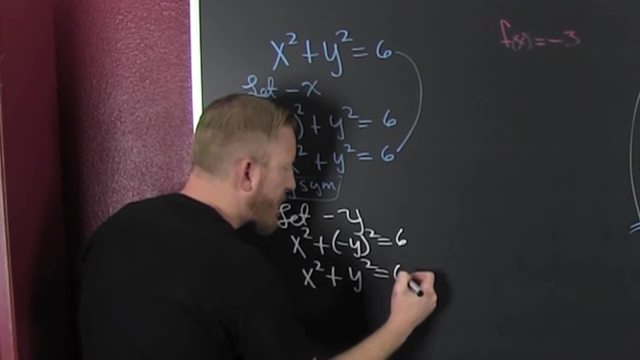 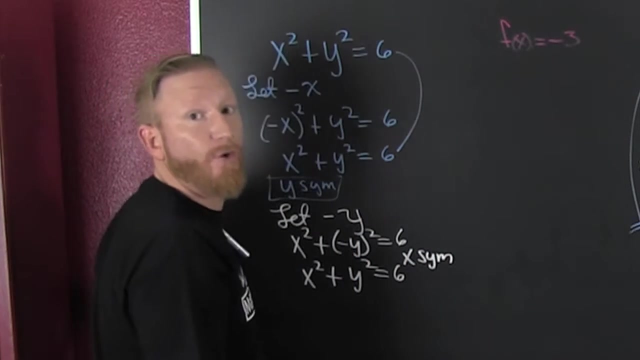 So that's x squared plus a minus y, squared is 6.. Again we get our original function. So this is x symmetric. To check origin symmetry: we let, we let. we let a minus x and a minus y. 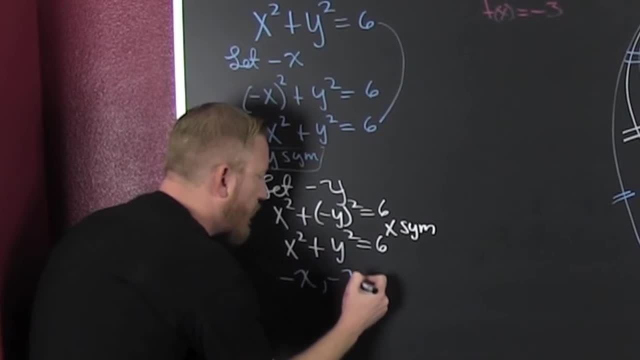 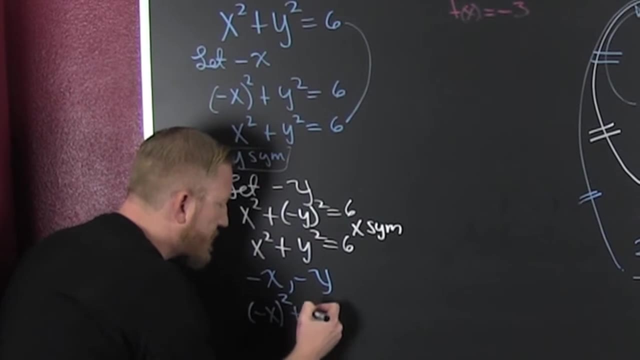 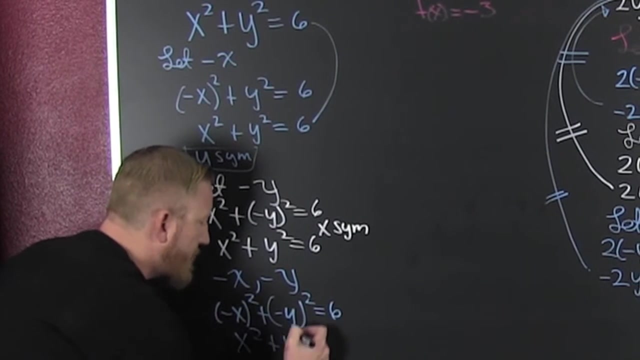 So a minus x and a minus y. When we let a minus x and a minus y up in there, we have a minus x squared plus a minus y squared. That's still equal to 6.. Wow, That's x squared plus y squared is 6.. 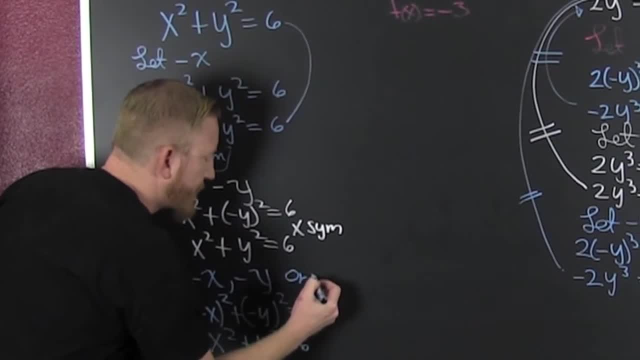 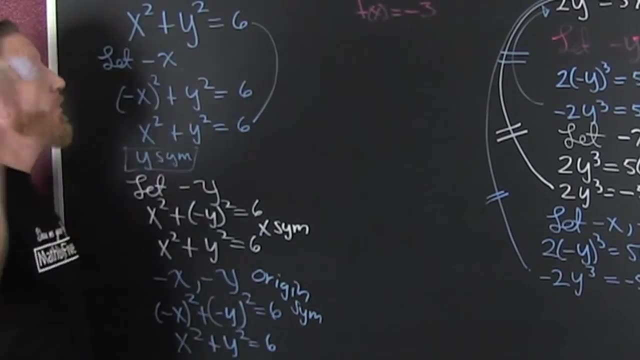 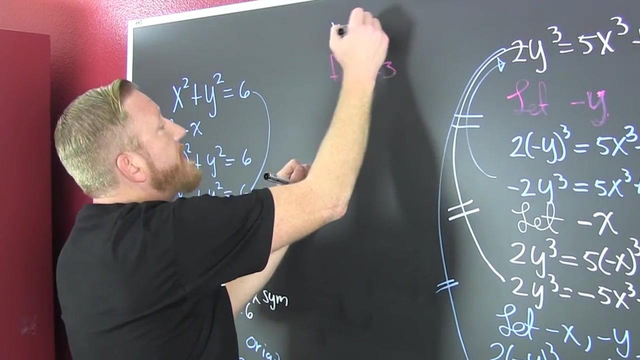 So this has all three times Great. What's next? Let's look at this. Okay, Great. What's next? This guy, Whoa, Fancy notation, What. What is that? That's, the function y is equal to a minus 3.. 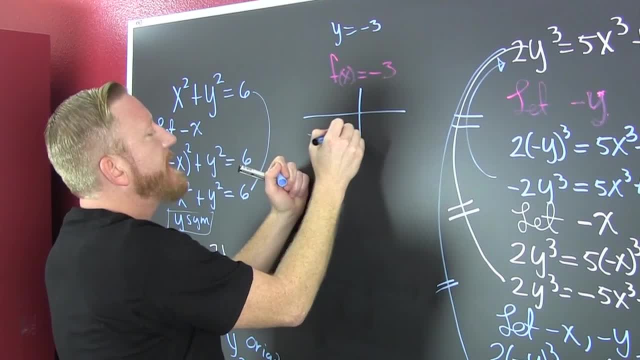 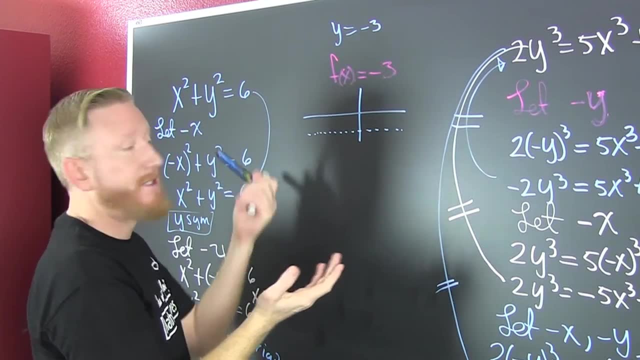 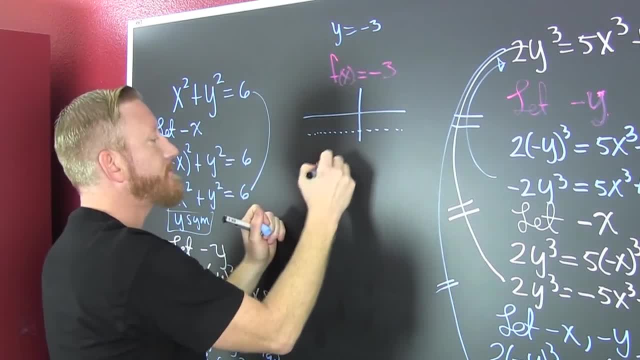 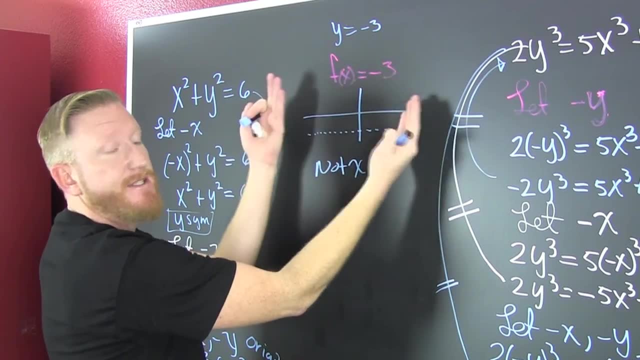 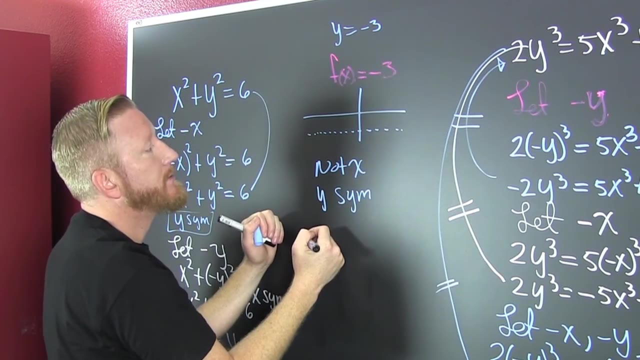 Is it a? No, It's not x. What about y? What about y? What about y? If I fold it across? y, is it the same on the left as it is the right? Yes, So it's y-symmetric. Now, what Origin? 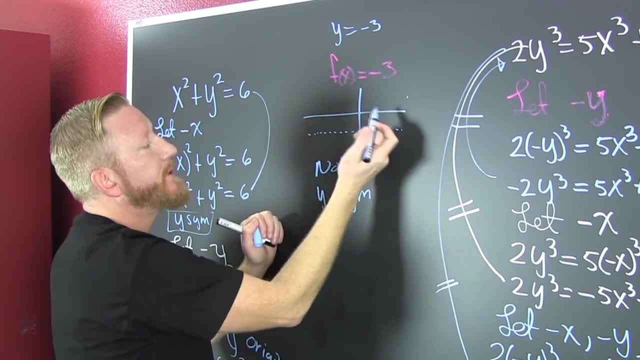 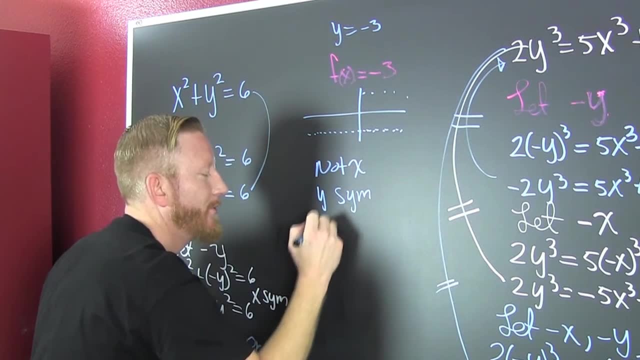 If I fold it on the y and then fold it on the x. so I fold it on y, bam, dot, dot, dot, dot dot, it's on itself. and then I fold: oh, no, no, no, no, no not.